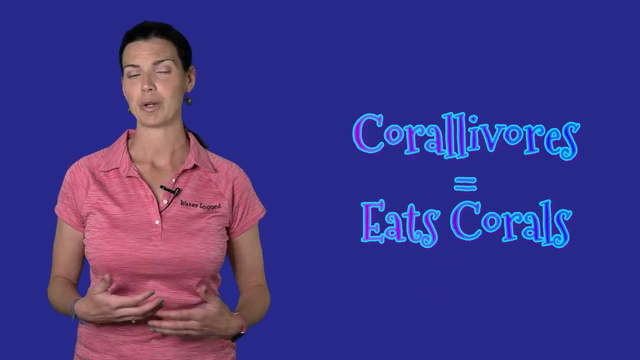 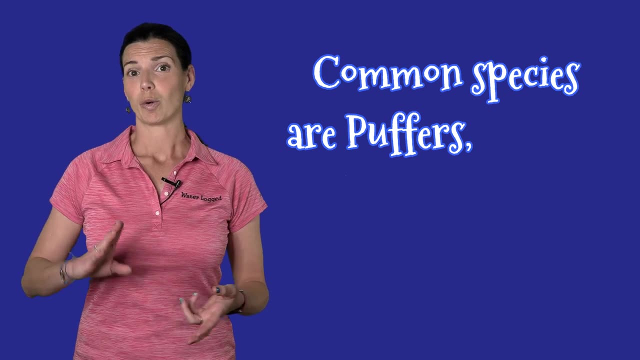 that the fish are typically in the wild eating corals, So you don't want to put them with any of those expensive corals that you want to buy for your tank. A lot of times these fish can be like puffer fish or trigger fish or even some of the larger predators, like 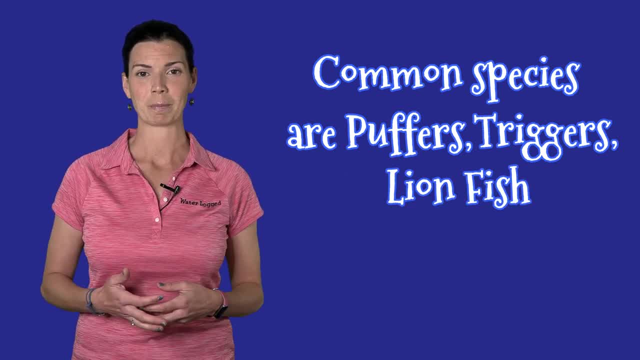 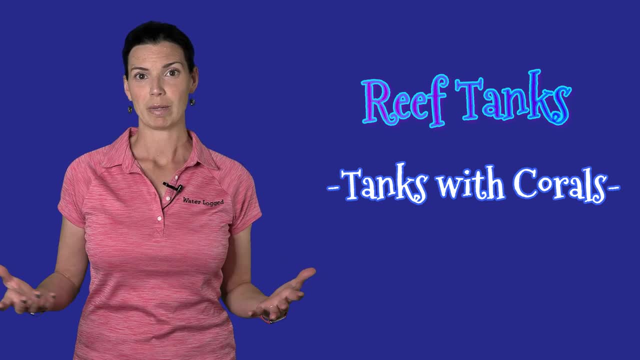 lionfish that you don't typically see in those reef tanks. Now let's move on to reef tanks. So reef tanks are any sort of tanks that might have coral in them. Now you can find these tanks in a variety of different sizes, So typically when you hear the word reef tank, 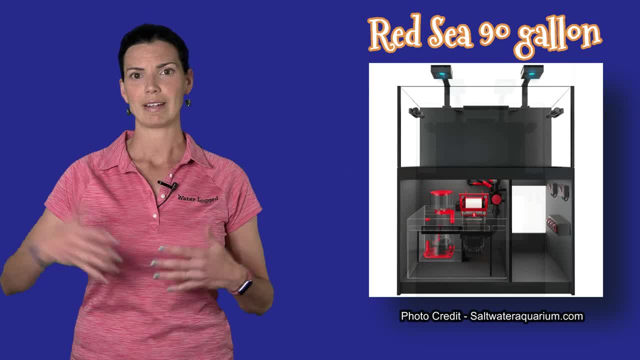 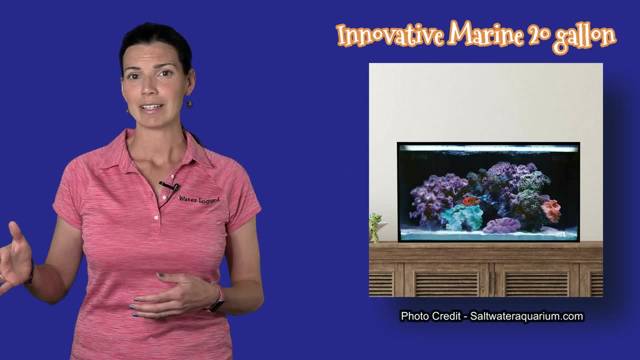 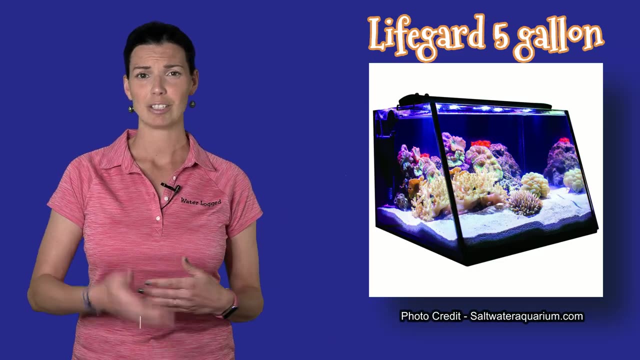 you're looking at anything, I would say, above a 40 gallon and up. Now you can also hear tanks referred to as nano tanks. I would say that's anything like 30 gallons, 30 or 40 gallons. You can also see a 10 gallon tank. Now, anything less than a 10 gallon tank is typically considered. 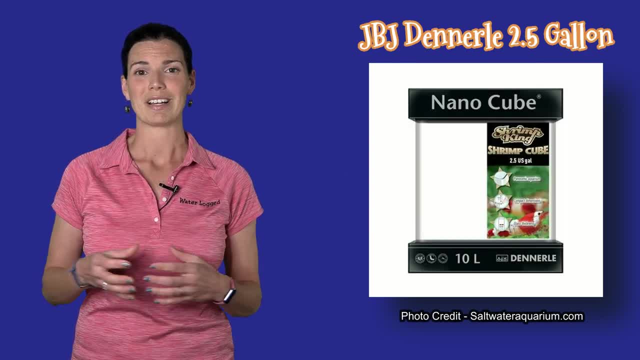 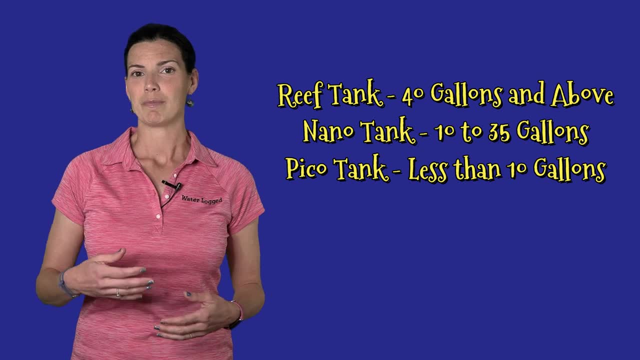 a pico tank. So those are the super, super small ones. So there's a variety of different tank sizes, but most of them, typically, are still going to have coral. Now, when it comes to coral tanks or reef tanks, you can have a bunch of different types of coral in the. 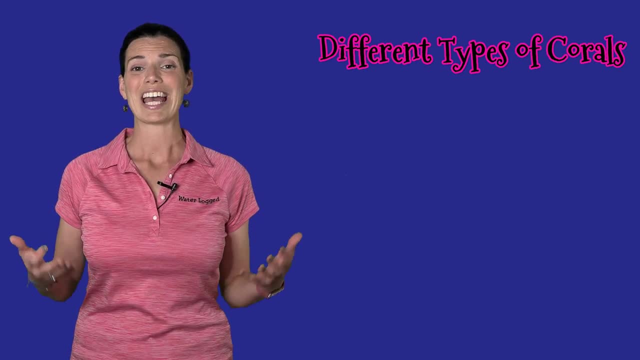 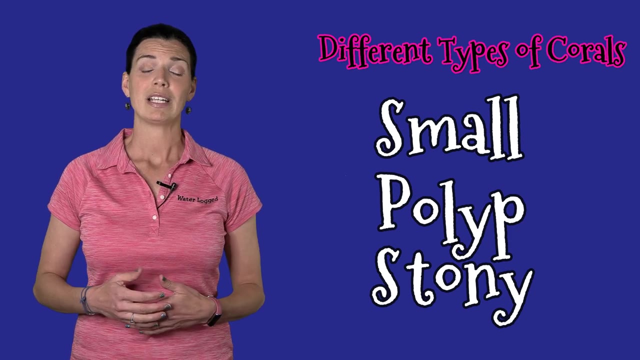 tank. So let's go over a couple of those. First off is SPS corals. Now, that stands for small polyp stony coral. Speaker 1. These species of corals are typically going to need a lot more light and a lot more flow. 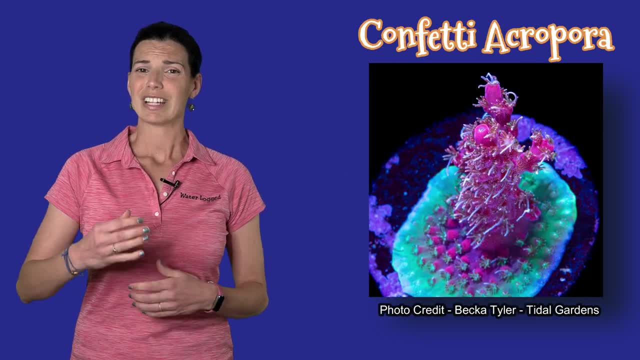 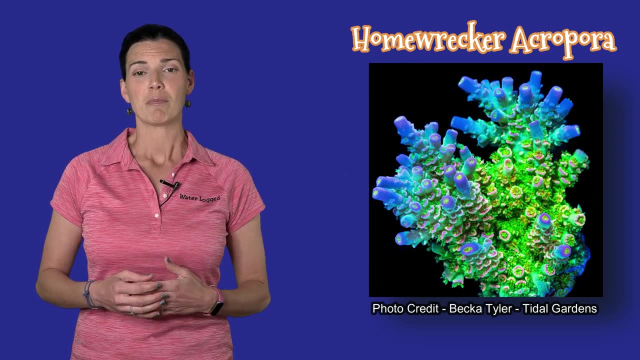 than the other corals that are on this list. Now, these aren't necessarily corals that I would recommend for beginners. A lot of times they're a good deal more sensitive to changes in water parameters, but they are some of the more sought after corals, especially. 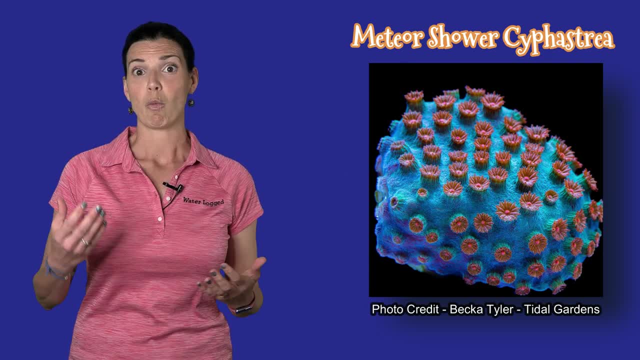 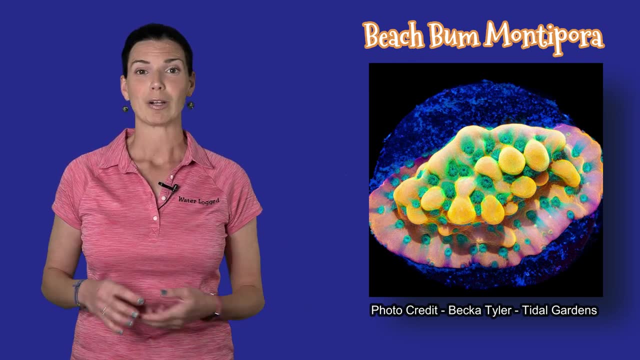 for long-term collectors. Now, if you're trying to figure out what corals are the SPS corals, you could have things like mataporas or some of the very popular active corals. Speaker 2. Speaker 1. You could have things like acroporas. They have things like the Walt Disney coral that. 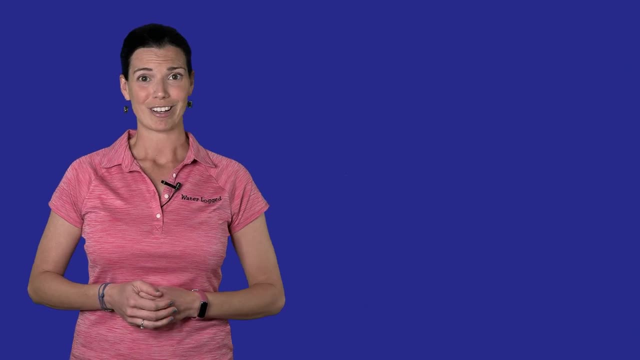 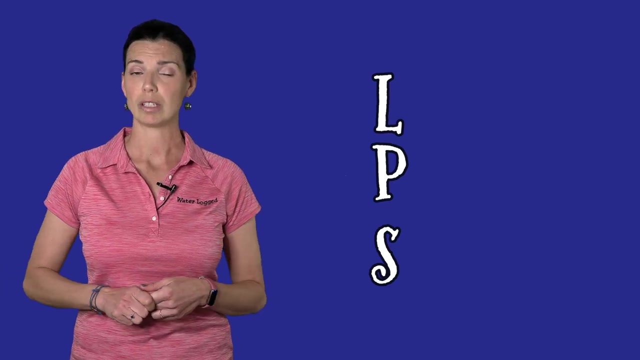 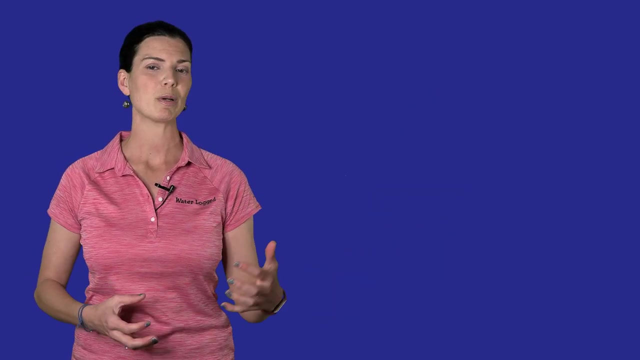 are just flowing with color and are very sought after. Okay, Now our next category of corals is going to be LPS corals. LPS stands for large polyp stony corals. Now, these guys, unlike the SPS corals, they're not going to need as much requirements when it comes to 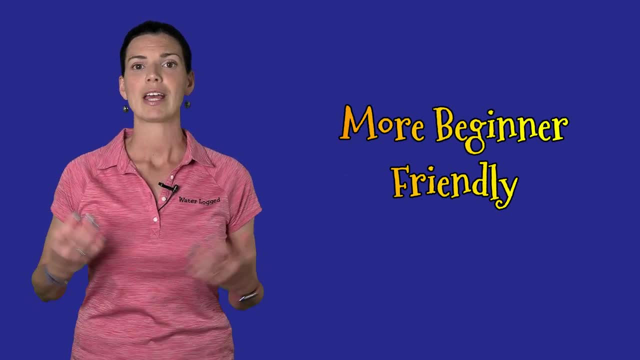 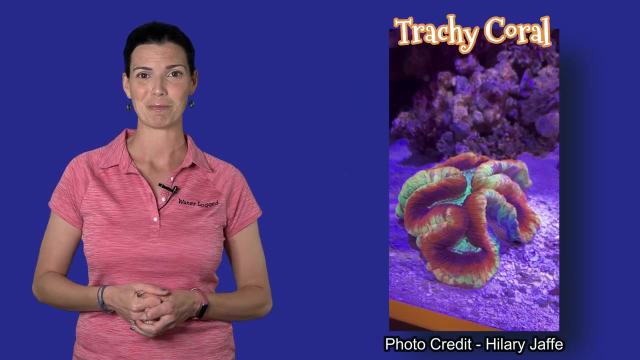 light and flow And when it comes to beginners, they're a lot easier for beginners to take care of. Speaker 2. So, if you are just starting out, these are the ones that I would recommend for you, And actually, LPS corals are some of my favorite. The first ones that I fell in love with are: 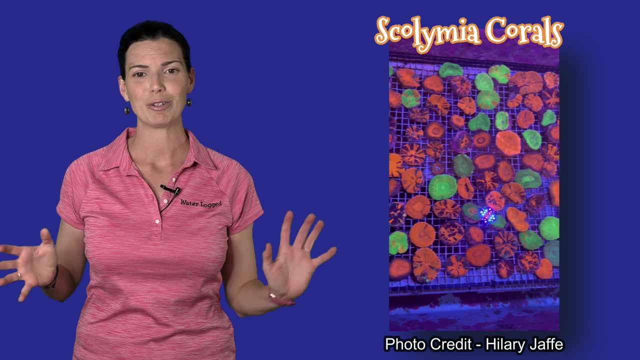 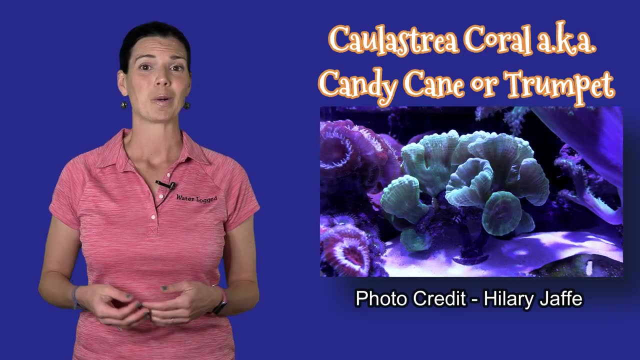 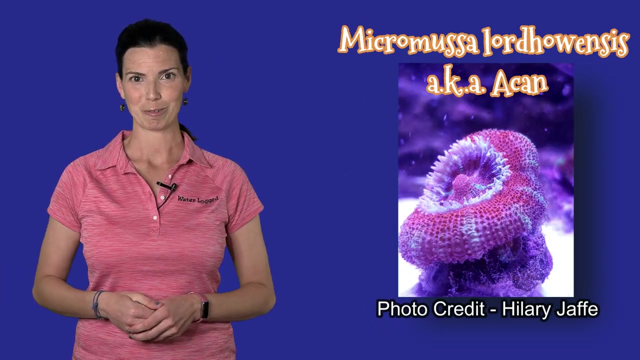 those scolies or scolimias. They come in amazing beautiful colors and they're so much fun to watch eat. But other ones are things like the candy cane corals or even things like those favias. So if you are a beginner, maybe stick towards those LPS corals. 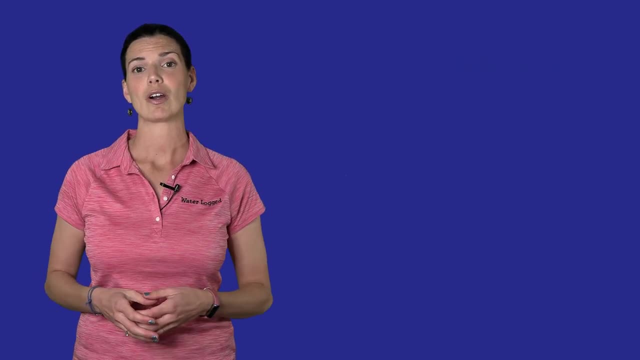 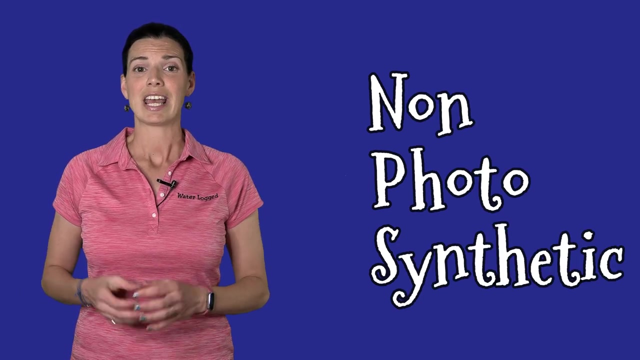 Speaker. 1. Speaker. 2. Speaker. 1. The next corals on our list are NPS coral. Now, NPS stands for non-photosynthetic. Unlike the other ones that we've talked about on this list, these corals don't have zooxanthellae. 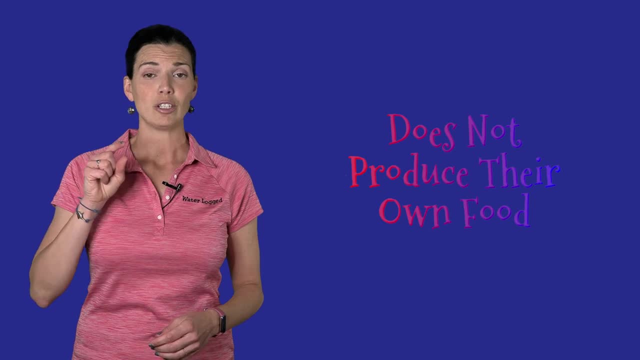 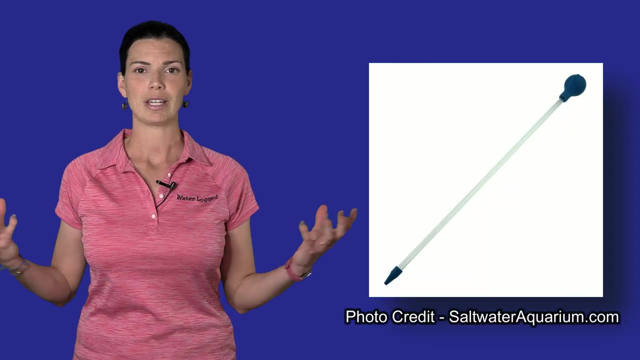 in them, so they're not able to produce their own food, which means that you're going to need to take a lot of care when it comes to making sure that they're fed. You can do things like target feeding, or you can do broadcast feeding, where you get the food dispersed throughout. 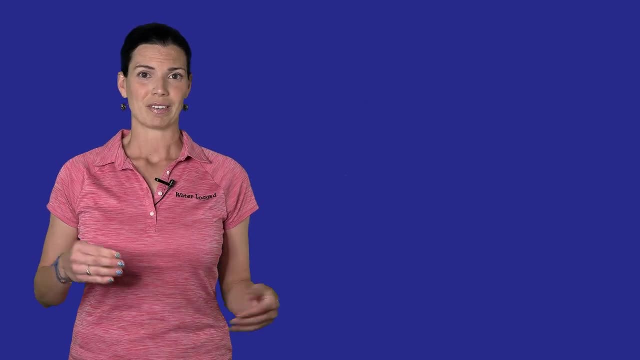 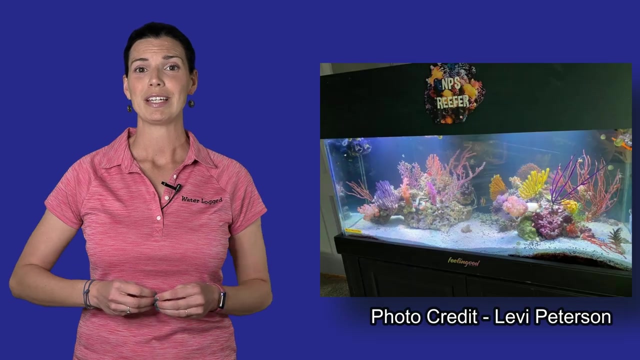 the tank, but food is really important for them. Now, these types of corals, the popularity of them in the aquarium community is just starting to grow and you can see more and more people that are keeping these corals, but they have things like the sun corals or 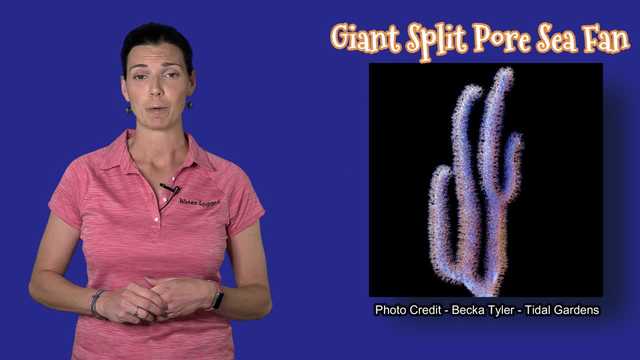 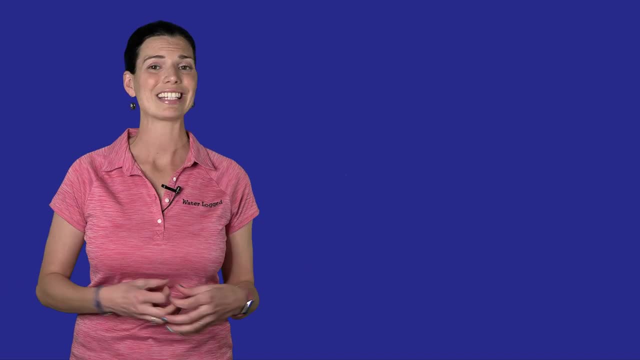 even the dendros, and sometimes you'll see sea fans in there. So if that is your cup of tea, then maybe look for some of those NPS corals. Speaker 1. Speaker 2. Speaker 1. Okay, Now our second to last group of corals is going to be our soft corals, or sometimes. 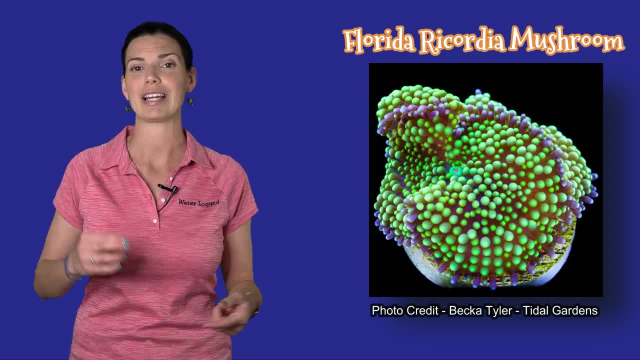 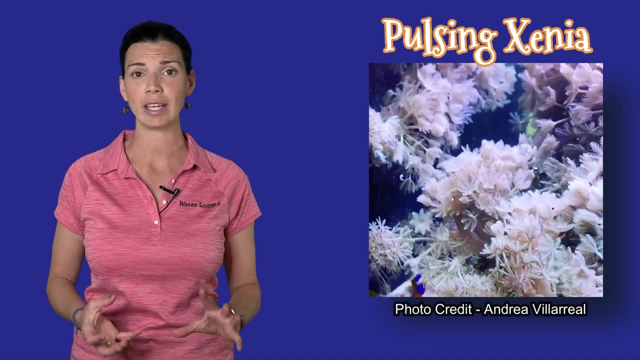 as they're referred to, softies. These include things like mushrooms and leathers, So if you're a corals fan, you might want to keep a lot of these. Now, these are great ones to keep if you are traveling a lot and don't have a lot of time to dedicate to your tank. These 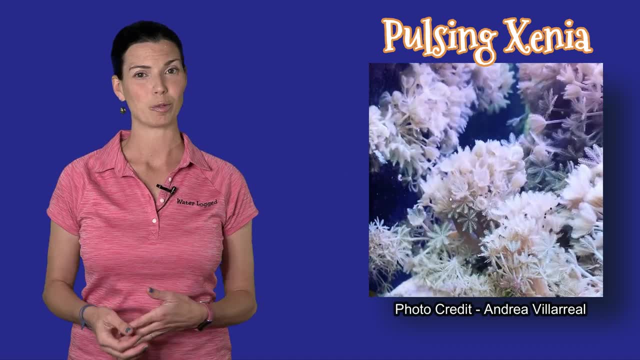 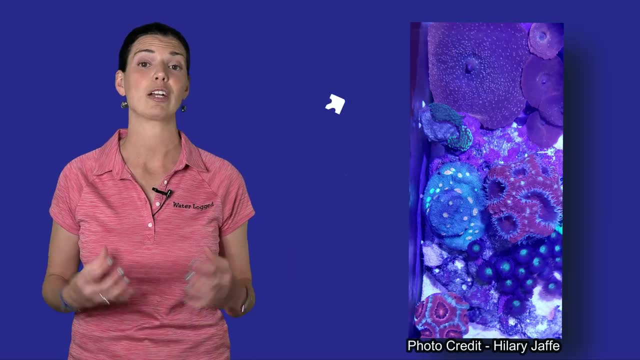 are relatively forgiving when it comes to mistakes and swings in water quality. Now, one thing I will warn you: with mushrooms especially, depending on the species, can actually take over a tank quite quickly. So you want to make sure that you at least keep. 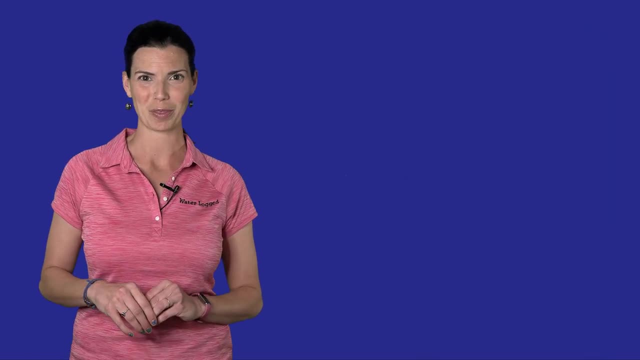 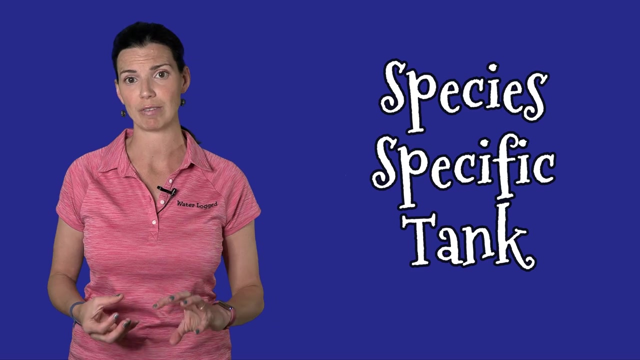 an eye on them and make sure they're not traveling around the tank where you don't want them. Speaker 2. Speaker 1. Okay, Now, the last type of saltwater tank that you might have when it comes to coral is a species specific tank.